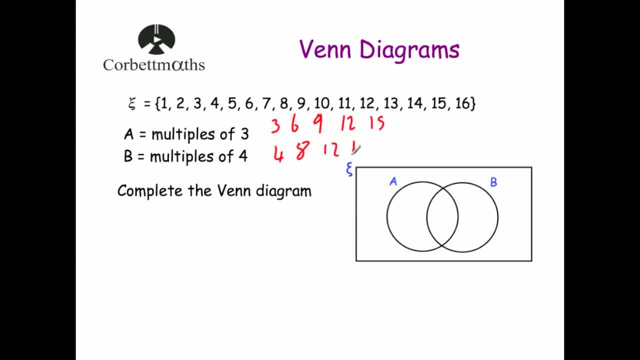 4,, 8,, 12 and 16.. And what we're going to do is we're going to put these into the Venn diagram. So let's first of all start off with the middle of the Venn diagram. So this: 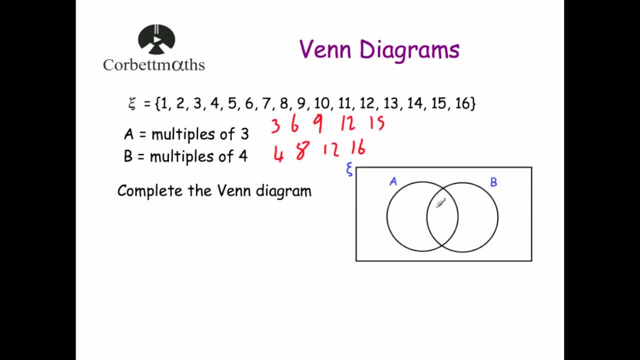 section here would be anything that's in a and in b, So it would be a number that's a multiple of 3 and a multiple of 4.. If you look above for this, 12 clearly satisfies that. So we're going to put 12 in the middle because 12 is a multiple of. 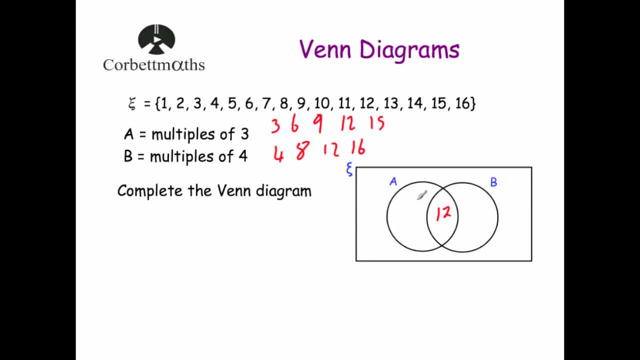 3 and it's a multiple of 4.. So it's in a and b. This section here would be anything that's just in a but not in b. Okay, so anything else, that's a multiple of 3.. So let's put our 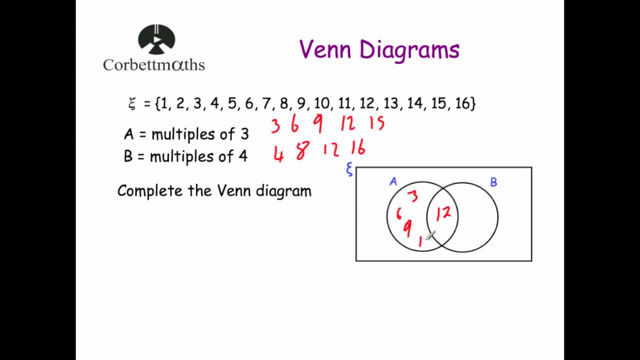 3, our 6, our 9 and our 15 in there. Okay, This section here, that would be anything that's a multiple of 4, but it's not a multiple of 3.. Okay, so that would be the rest of the multiples. 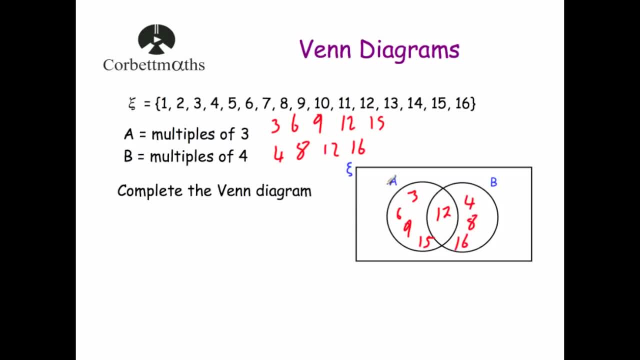 of 4.. So that would be 4,, 8 and 16. And around the outside that would be any other number that we haven't got in the diagram so far, So anything that's not a multiple of 3 or a multiple of 4.. So let's put in our 1, 2, we've got 3, 4, then that would be 5, we've got 6, 7.. We've got 8,, 9,, 10,, 11,, 12,, 13,, 14,, 15,, 16,, 17,, 18,, 19,, 20, 21,, 22,, 23,, 23,, 24,, 24,, 25,, 25, 26,. 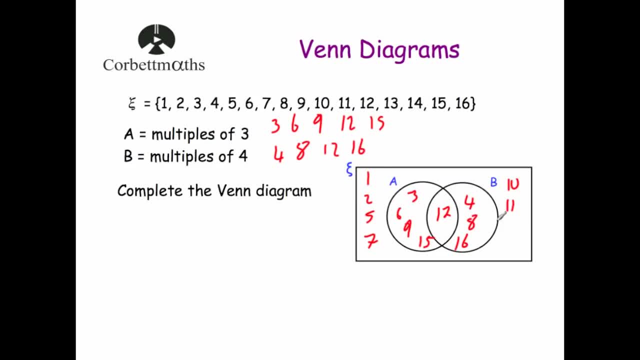 27,, 28,, 30,, 32,, 33,, 35,, 36.. We've got 8,, we've got 9,, 10,, 11,. we've got 12,, 13,, 14,. we've. 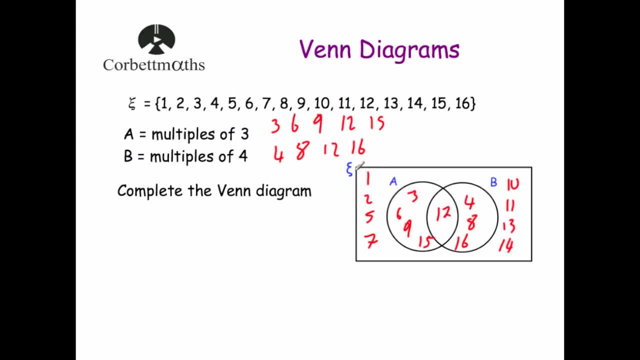 got 15, and 16.. That's it. But whenever you're doing a Venn diagram question, I always recommend you check you've got all the numbers or all the data. So let's, we've got the numbers 1 to 16, so we've got 16 numbers. So 1, 2, 3, 4, 5, 6, 7,, 8,, 9, 10,, 11,, 12,. 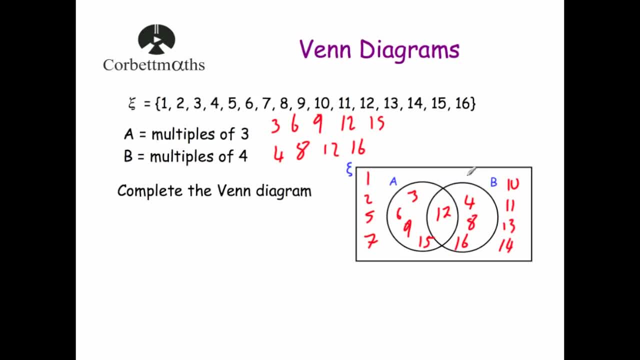 13,, 14,, 15,, 16.. So we've got 16 numbers in there. so that's it. we've completed the question. So that's a Venn diagram. okay, It's how you, it's quite straightforward, You could. 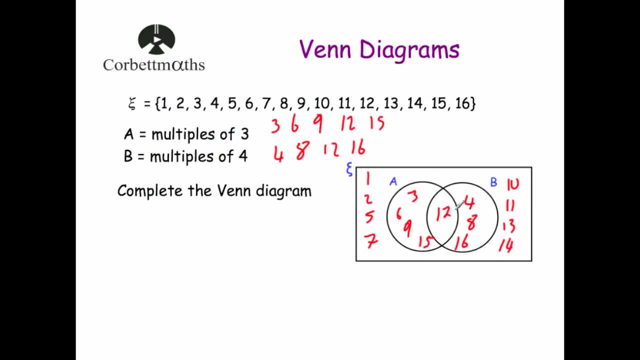 it's quite straightforward. venn diagram question. uh, we've put in the numbers in a, the numbers in b, the middle section where they overlap. so anything that's in a and b and anything on the outside is anything that's not a or b. okay, let's have a look at another question. the venn diagram shows: 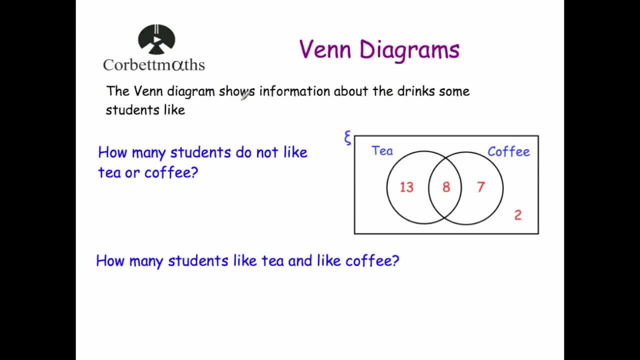 information about the drinks that some students like. okay, so some students were surveyed and this is the type of drinks they like. the first question says how many students do not like tea or coffee. okay, so if you can see here, the first circle, here is anyone that likes tea. so these 13 people and 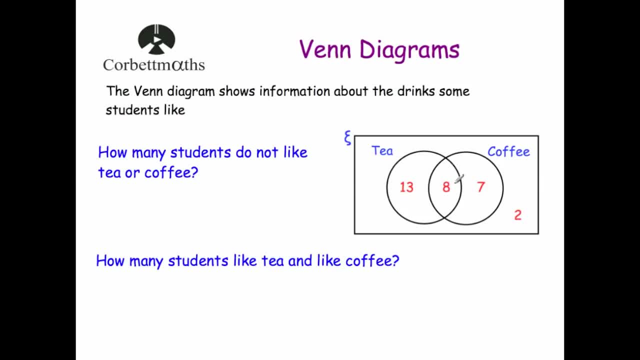 these eight people all like tea. the eight, well, it's both tea and coffee. so these eight people like tea and coffee because obviously they're in both circles. this is these seven here. they just like coffee, but they don't like tea. and the two people outside, well, they don't like tea or coffee. 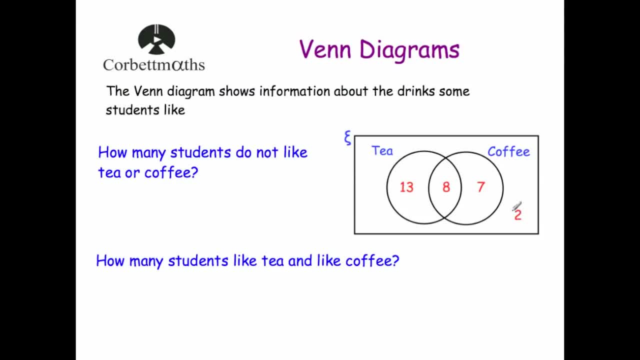 so the first question says how many students do not like tea or coffee? well, it's going to be these two students here, so it's going to be two. next question says how many students like tea and coffee. so because- and it means they like tea and coffee- it's going to be the people in the middle that. 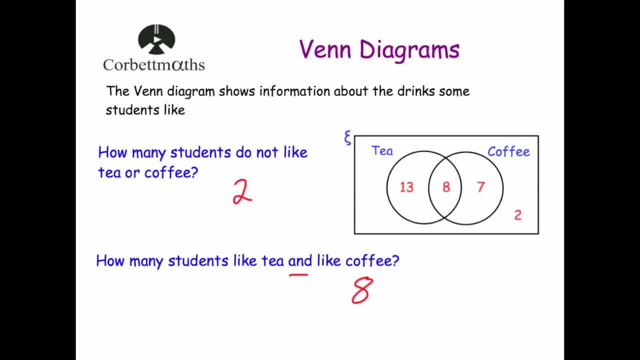 like tea and coffee. so there's eight students that like tea and coffee. next question: how many students like tea? well, obviously we've got these two uh numbers here. we've got our 13 and our eight and they're both in the circle for tea. so if we add them together we'll see how many people like. 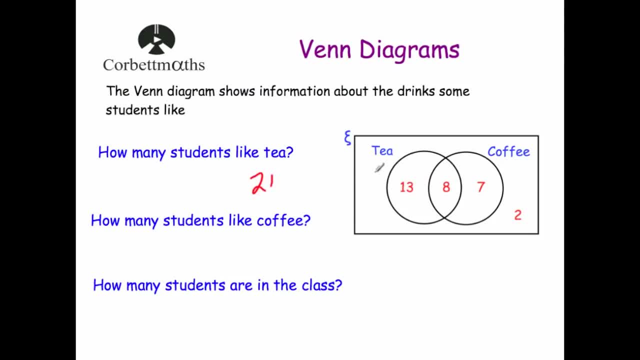 tea. all together, well, 13 plus 8 is 21, and that's it says how many people like tea. we've got the 13 people that like just tea, and we've got the eight people that like tea and coffee. so all together there's 21 people that like tea and coffee. so we've got the eight people that like tea, and 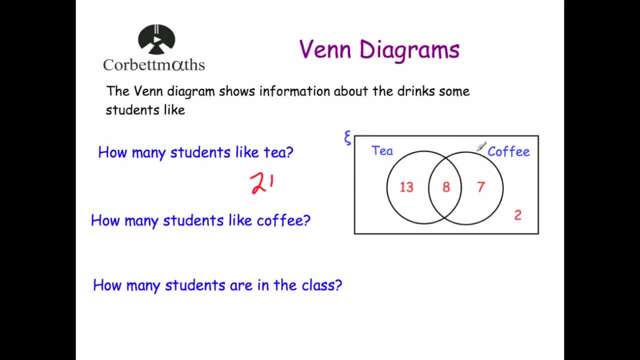 tea. the next question says how many people like coffee. so if we look at the coffee circle, we've got the eight and the seven inside. if we add them together, there's 15 people that like coffee all together. the next question says how many students are in the class. well, if we add all the numbers, 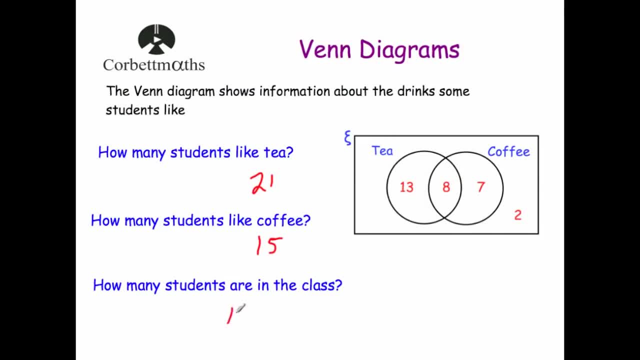 together. in the venn diagram we'll see how many people are in the class. so we've got 13 plus 8, which is 21, plus 7, which is equal to 28, plus 2, which is equal to 30, so there's 30 people in the. 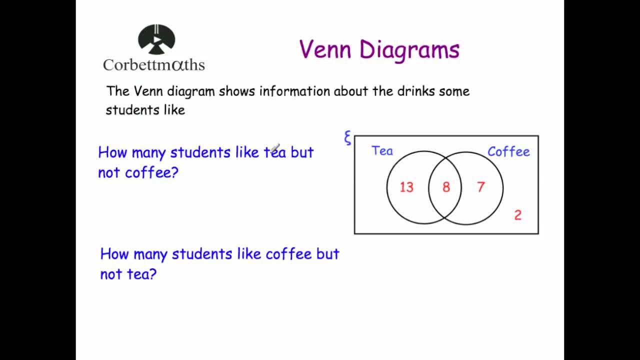 class. next, how many students like tea but not? uh, but they do not like coffee. okay, so the people that like tea and not coffee would be these 13 people here, because they're in the t circle but they're not in the coffee circle. okay, so it'd be 13.. and the next person says how many students 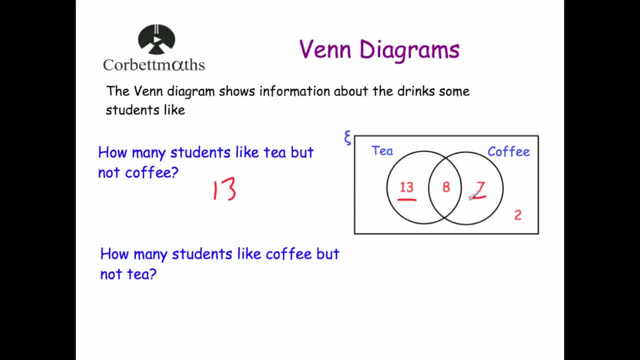 like coffee but not tea. well, if you look at the coffee circle, that'd be the seven. seven people like coffee but not tea. so the the. we're sort of getting used to sort of reading venn diagrams and understanding how to approach, understanding what the numbers mean. okay, so 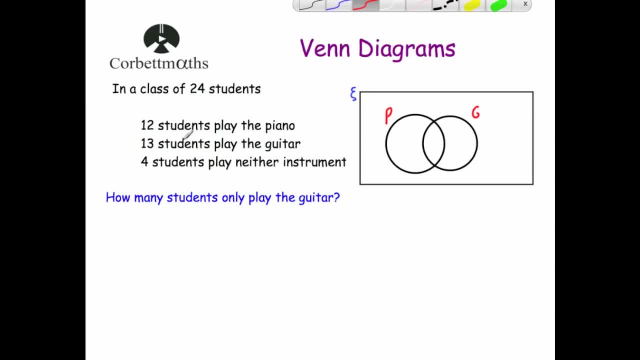 the next example says: in a class of 24 students, 12 played the piano, 13 students played the guitar and four students play neither instrument. so what we're going to do is we're going to fill in the venn diagram to begin with, and then we're going to be able to answer the question: how many students? 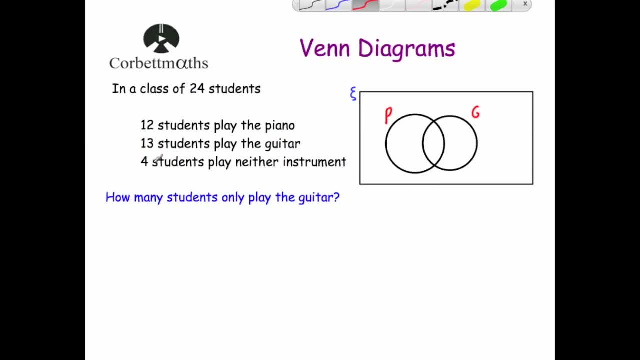 play the guitar only. okay. so first of all let's put the four students that play neither instrument outside. now this: 12, the play the piano, that's the whole circle. okay. and 13, the play of the guitar, that's the whole circle here. okay. now we don't know which numbers in the 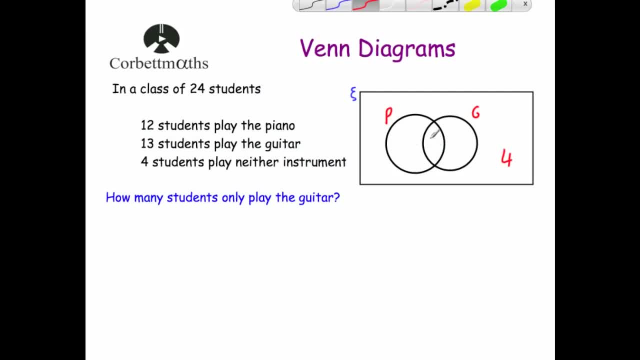 middle. so we can't just quickly fill out these three numbers, but what we we can actually from the information we've been given, because we know there's 24 students all together. we can use one of the numbers. so let's just look at the 12 and we know that in the piano circle this whole 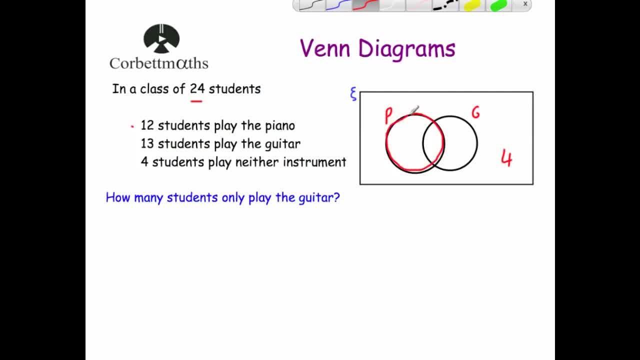 circle here. we know that there's going to be 12 students, so let's just put a 12 in there for now, okay. and we also know the four play play neither instrument. so we know there's 12 there and there's four there. now that's 16.. now, all together, there's 24 students. 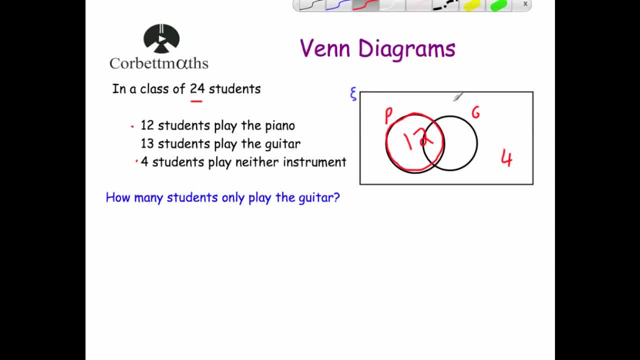 now, there's only ever going to be four numbers to add together in this, in this question, we've got, uh, these two here, this one and this one, but they're 12 all together, the one that we don't know and the four, so we do 12 plus 4, that's 16.. well, if we add on it, we're. 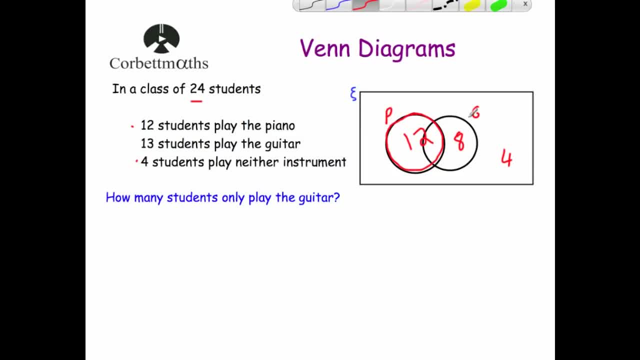 going to get the 24.. so that means that this section here, the bit that's only guitars here, actually answers our question. it let's just fill in the rest of the venn diagram anyway. okay. so let's rub out the 12 now and let's work out the two other numbers in the venn diagram, okay, the. 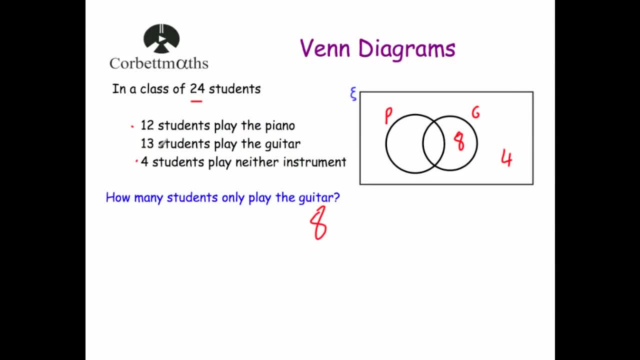 bit in the middle and the bit in the middle and the bit in the middle and the bit in the middle. this piano. only now we know that 13 play the guitar, so that's a whole circle here. now if there's eight there, that means that the five is in the middle to make 13.. so because five plus eight, 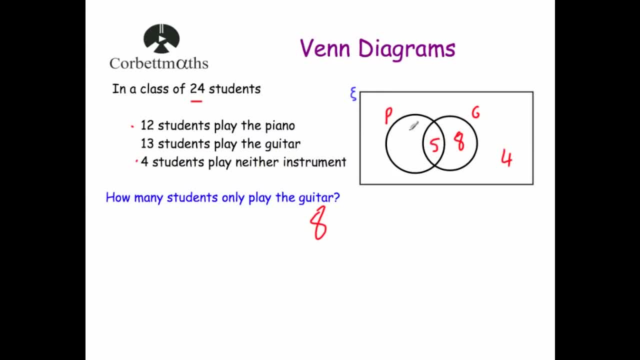 is 13.. now we know it's five in the middle and we know that 12 play the piano. that's this whole circle. here is 12. if we notice five there, that's going to put seven on that side. that's it. we've filled in the venn diagram and just to go through the question again, it says how many students only. 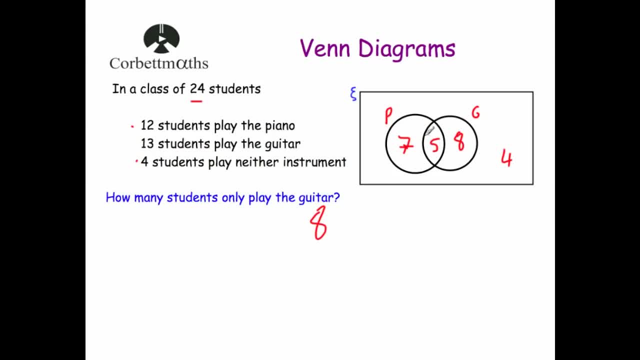 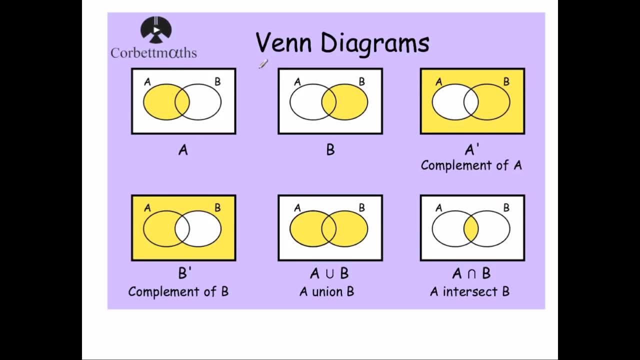 play the guitar. well, that's the uh, the guitar circle, but the bit, and it's not in the middle. so that's it. that's it. we're now going to look at some notation that you might encounter whenever you're doing a venn diagram question. so we've already seen a, okay, so 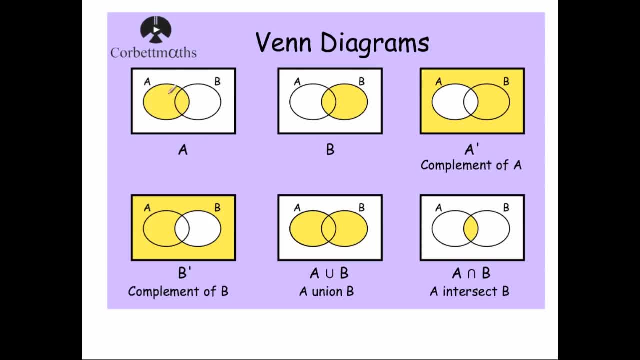 if you have a circle here in the venn diagram that's labeled a, anything inside it would be part of the set a. uh, next, inside of b is obviously b, now an a with a, a dash like this: that means the complement of a. all right, that means not a, so it means anything that is not inside the a circle. 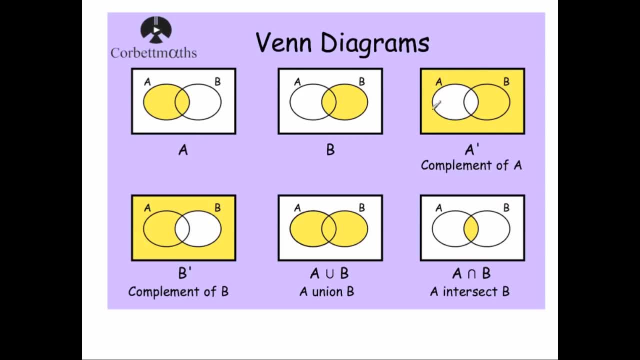 so well or oval in this question. so here you've got the circle of the region for a. anything outside of it would be a dash, which is the complement of a. likewise b dash, that would be the complement of b. so anything outside of b- now a and this u and then b- means a union b. 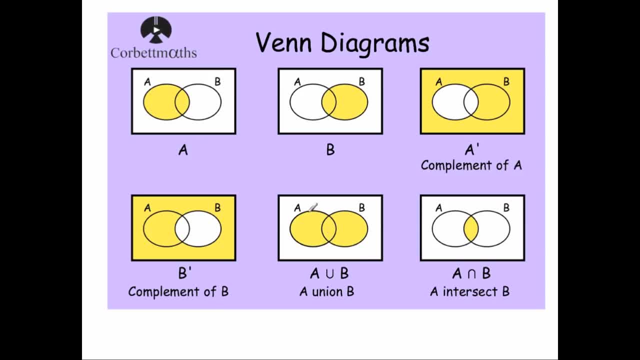 and that means anything that's an a or b, all right. so anything in the a circle or the b circle would satisfy or be part of the group or the set a union b. so a union b is anything in a or b. i like to sort of consider the word or whenever i see that. 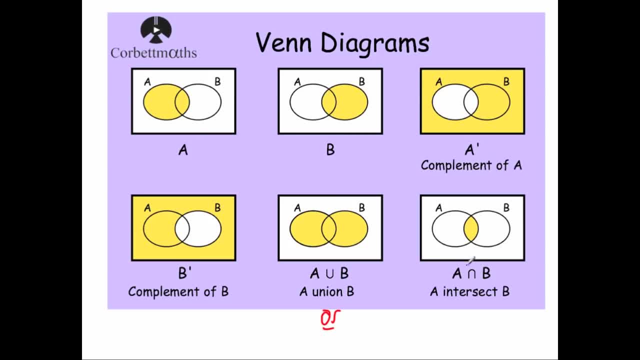 and so finally a and then an n and then b. it's not like a an n, it's like a. it's the shape. okay, the symbol a. the symbol b would be a intersect b. it means anything that's in a and b. okay, so nf. it would be in the middle region. okay, so a intersect b is anything that's a and b. okay. 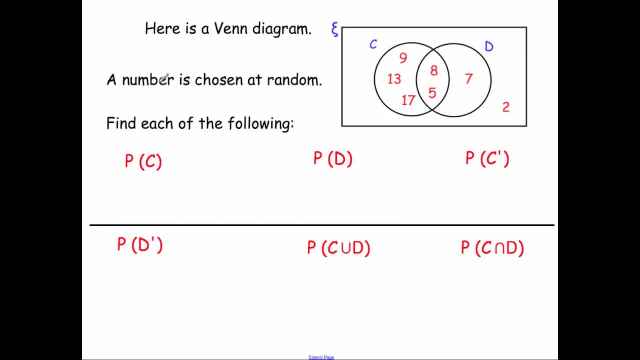 let's have a look at some questions. so here's the venn diagram. a number is chosen at random from this venn diagram. find the probability of each of the following. so let's see how many numbers in the venn diagram to begin with. so we've got one, two, three, four, five, six, seven. so seven numbers and 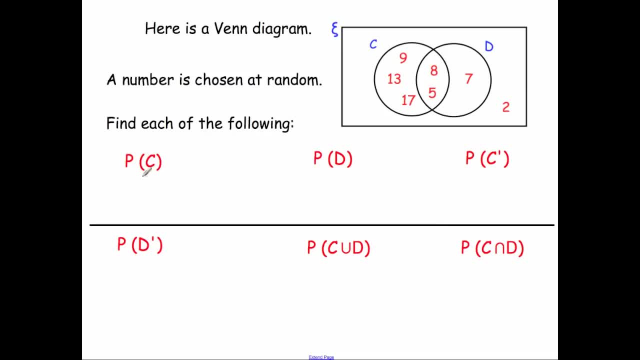 the first one says: what's the probability of uh forgetting c or uh, what's the probability? the number chosen is from c, so there's one, two, three, four, five and c, so it's gonna be five out of seven, probably if d. well, there's one, two, three numbers in d, so that'd be three, sevenths. 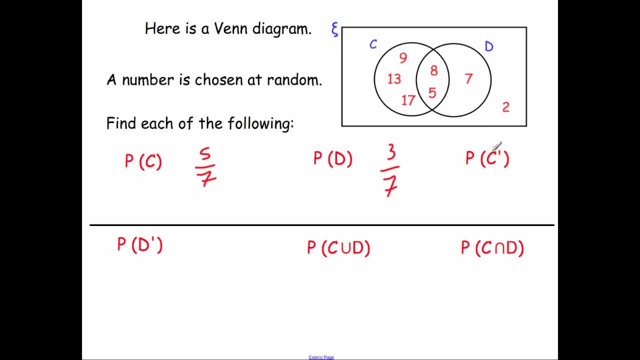 the probability, if the complement of c or a probability of c dash means the probability of not c. so it means: what's the chance of picking a number that is not in c? so we've got five numbers in c, but these two numbers, the seven and the two, are part of c dash, or 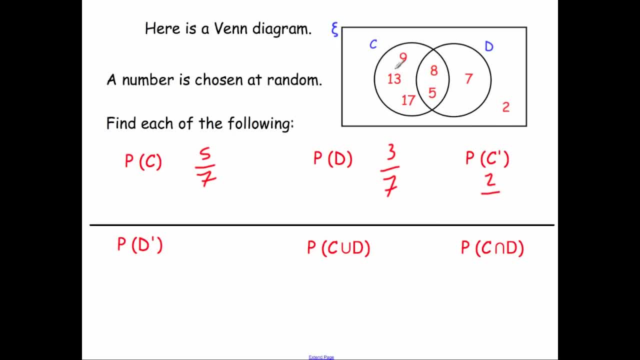 the complement of c, so it's going to be two out of seven. next, the probability of d dash. so that means this: the probability of the complement of d or any number that's not in the d circles. there's one, two, three, four that's not in the d circles, so it's going to be four out of seven. 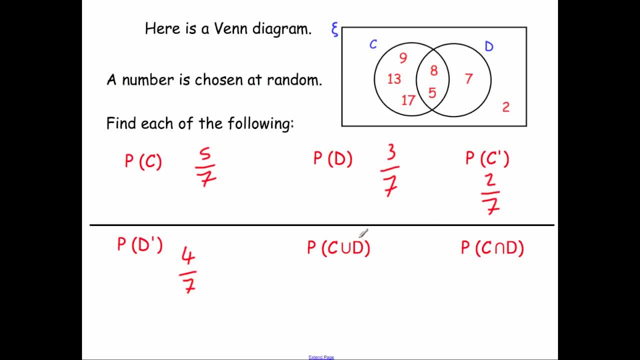 next one: what's the probability of c union d? so the pro c union d is anything that's in c or d. so there's one, two, three, four, five, six numbers in the c or d circles, so it's going to be six, sevens. and finally, what's the probability of c? 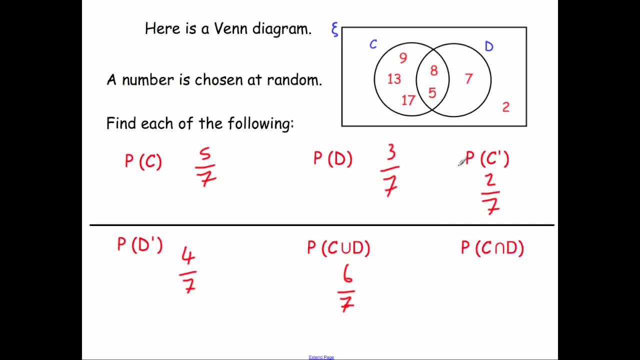 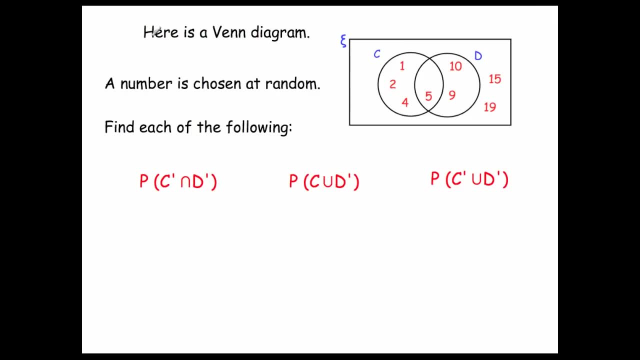 D, In other words the middle region, anything that's in C and D. So there's two numbers there, so it's going to be 2 out of 7, two 7s, Right? so our second, last example. Here's a Venn diagram and a number is chosen at. 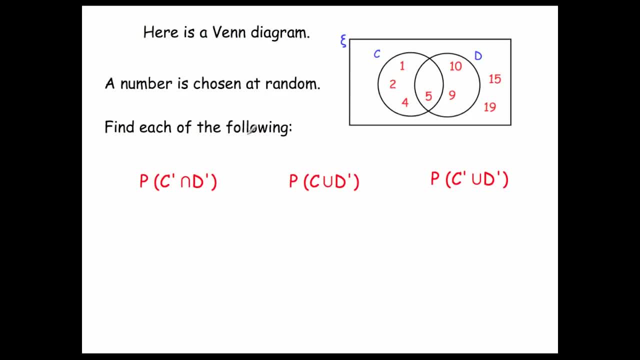 random. from the numbers in the Venn diagram, Find the probability of each of the following. So the first one: what's the probability of the complement of C intersect the complement of D? In other words, what's the probability of not C and not D? Well, there's one, two. 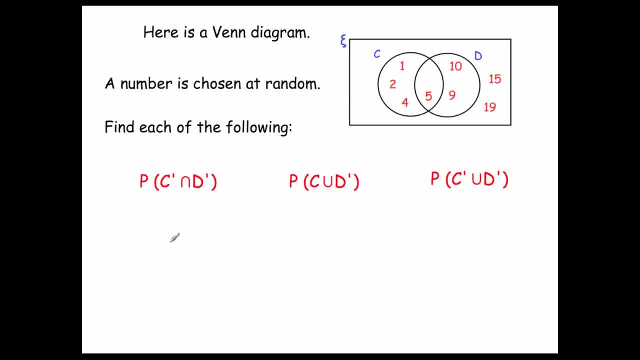 three, four, five, six, seven, eight numbers in this Venn diagram. so it's going to be eight in the denominator and not C and not D. well, that's going to be the two numbers on the other side. so that's going to be two eighths or one quarter. 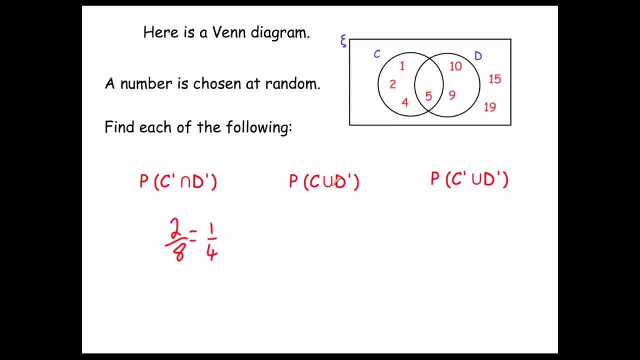 Next, what's the probability of C union, not D? So that means what's the probability of C or not D? So that means that anything that's in C or not D will satisfy it. So C will be these four numbers and not D. 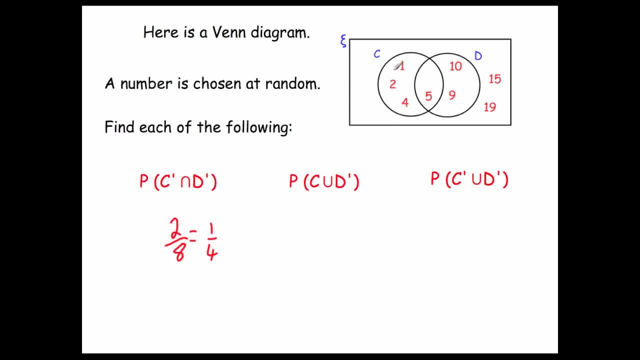 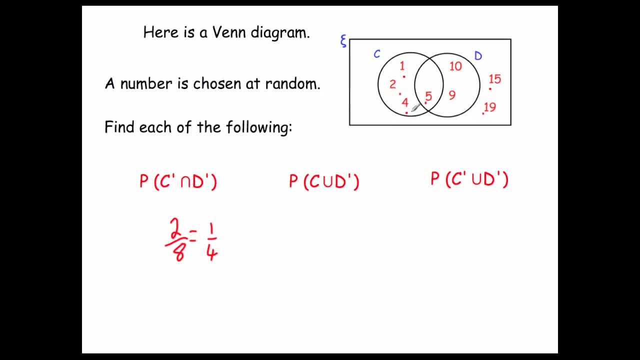 that we're going to accept any of them. So it's going to be anything in this circle or anything outside of the D circle. So the only two that we're not going to be looking at will be the ten and the nine. So it's going to be six over eight, and that's equal to. 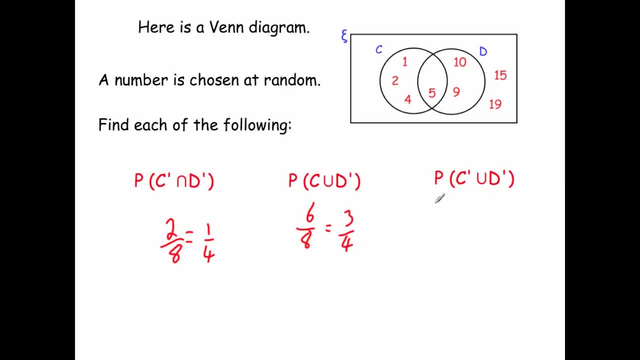 three quarters Right. so the last part of this question says: what's the probability of C union, not D? Well, the probability of the complement of C union, the complement of D, In other words, what's the probability of not C or not D? Now, because it's union, it means that it's either one. 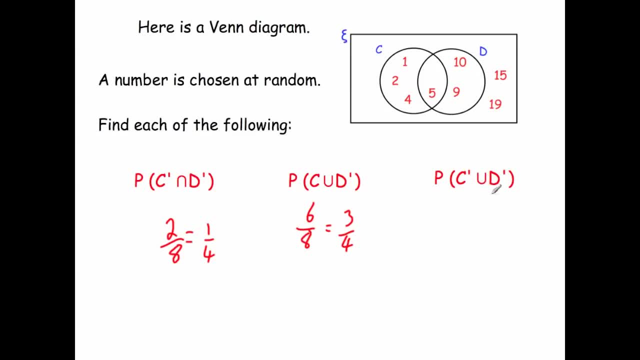 of them. Okay, so if it's not C or not D, then it's part of it's accepted. So not C. Well, not C. let's take it would be that number, that number, the ten, the nine, the fifteen. 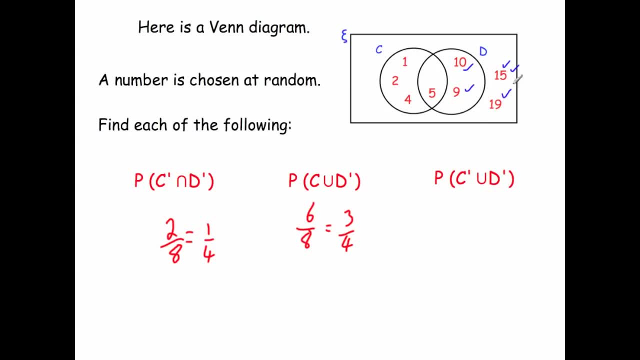 or the nineteen, Not D. well, not D would be the fifteen and nineteen again, but also the one, the two and the four. So the probability of not C or not D would be any of the numbers that we've ticked. So 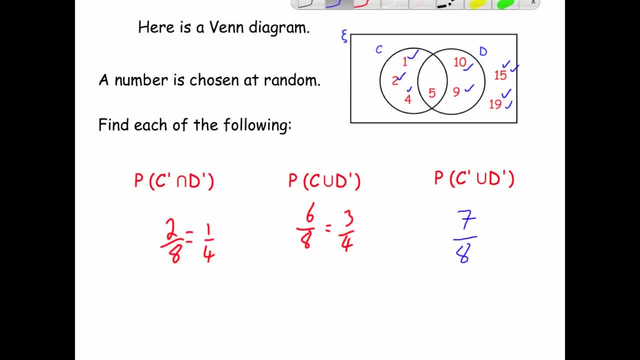 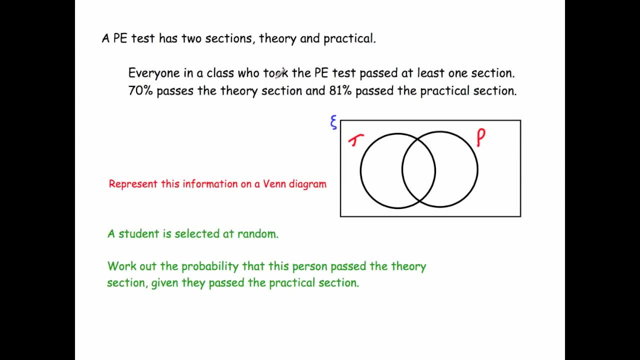 it's going to be seven over eight And our last question. So the last question says a P test has two sections: a theory test and a practical test. Everyone in the class who took the P test passed at least one section. So it means that everyone's passed at least either the theory or the practical. 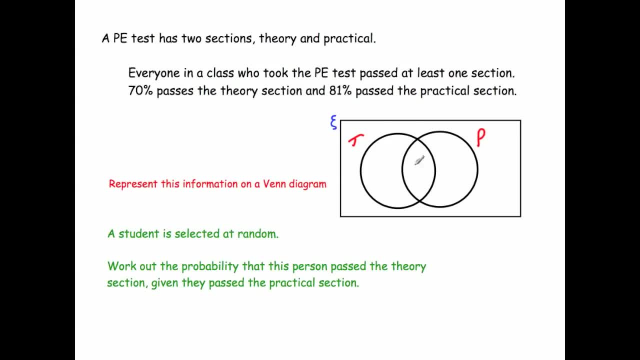 or both. It says that seventy percent passed the theory section. So in other words, we know there's seventy percent in this circle. There's going to be seventy in here, So we're going to have eighty one percent passed the practical section. So we know there's eighty. 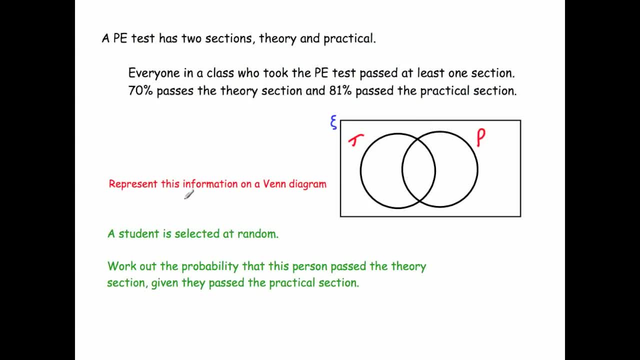 one in this circle And it says: represent this information on the Venn diagram. Now, to begin with, we know that nobody failed both sections, So let's put zero on the outside. Now this might seem a bit difficult because we don't have very much information to find. 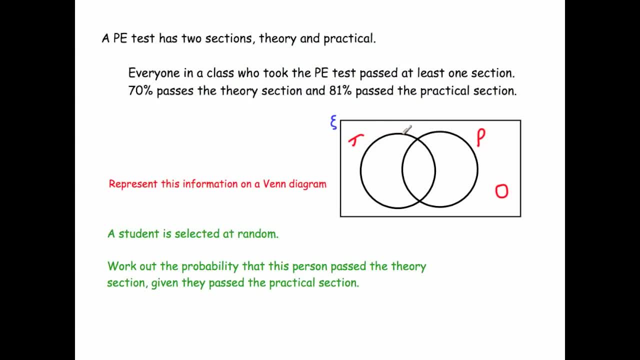 out what's in the middle. but actually we do have enough information. We know that there's four numbers altogether in this Venn diagram that we would have. We'd have this number, this one, this one and the zero. All right,